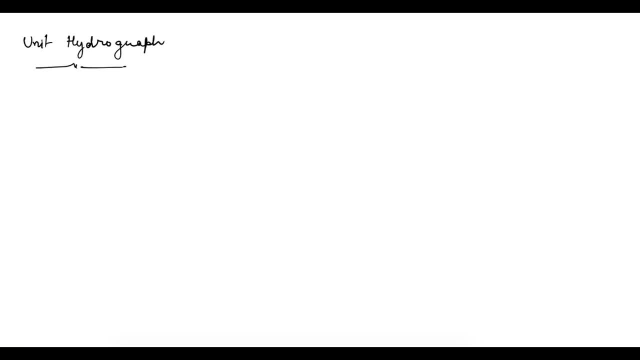 Hello everyone. Till now we saw the theoretical part of unit hydrograph. What is a unit hydrograph? It is a direct run of hydrograph resulting from a rainfall axis of 1 centimeter and this unit hydrograph would be corresponding to a particular DR duration. and we saw there are some assumptions. 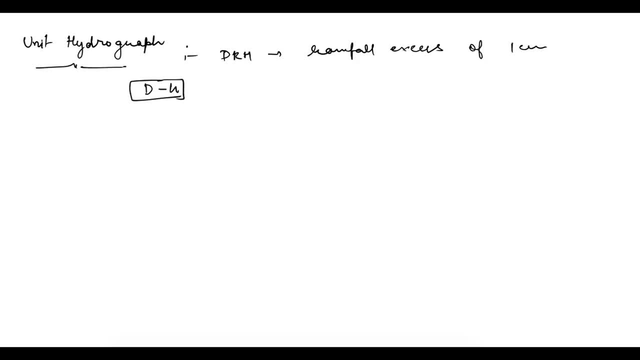 involved, like intensity is uniform and the precipitation will be uniform over the catchment. and two other assumptions were time invariance and linear response. So with the help of this unit hydrograph and with the help of these assumptions which are involved, we can solve some questions or we can solve some problems. So two types of problems can be solved, that is. 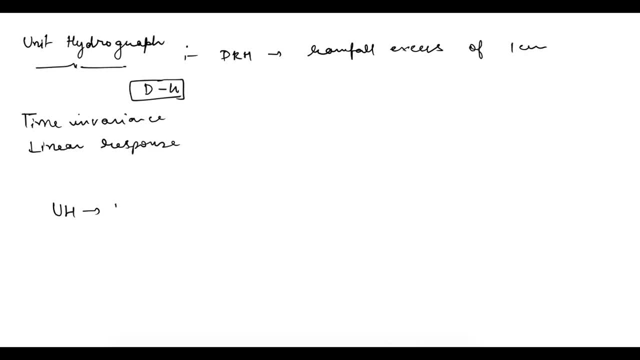 first is if you have been given the unit hydrograph for a particular DR duration so you can obtain the direct run of hydrograph. So if you have been given the unit hydrograph for a particular DR duration for the same DR duration, So unit hydrograph will be corresponding to 1 centimeter of rainfall. 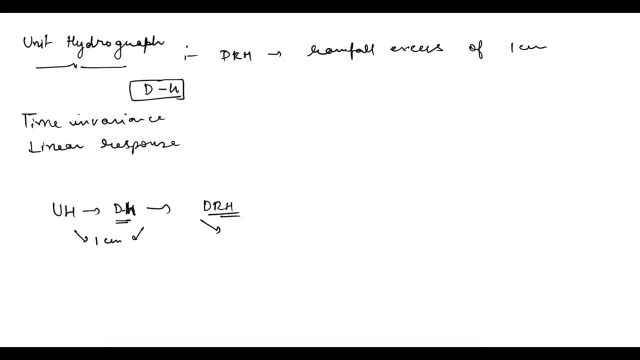 axis, so we can obtain a direct run of hydrograph which can be corresponding to any x centimeter of rainfall axis, and if base flow is also given, then we can obtain the flood hydrograph also, or hydrograph as we call it, that can also be obtained by, I mean doing the addition of this- 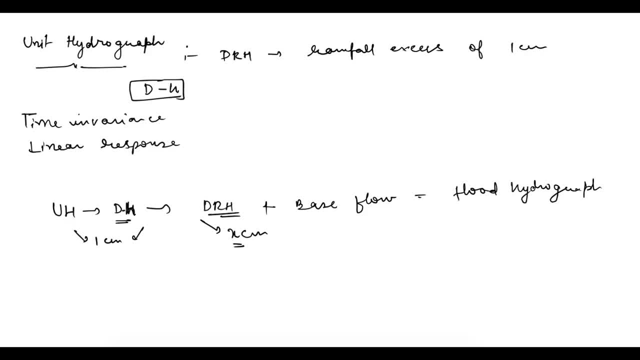 runoff hydrograph and base flow. So this we will see a question for that. Second type of problem can be: if you have been given the direct runoff hydrograph, So from that to obtain a unit hydrograph, So this direct runoff hydrograph will be for a particular DR duration and so 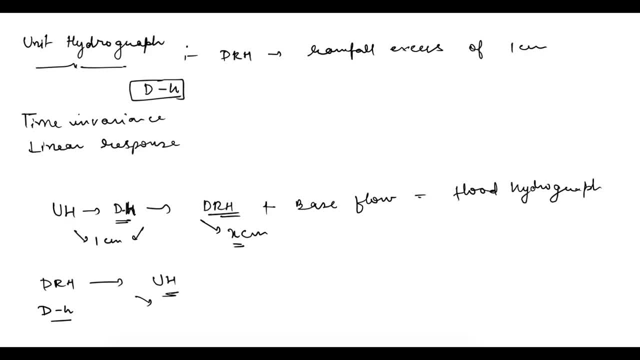 for the same duration, unit hydrograph can also be calculated. So for that we will have to find out that this direct runoff hydrograph is corresponding to what rainfall axis. So if we know the rainfall axis, then we just have to divide the ordinates or discharge by this rainfall axis to obtain the 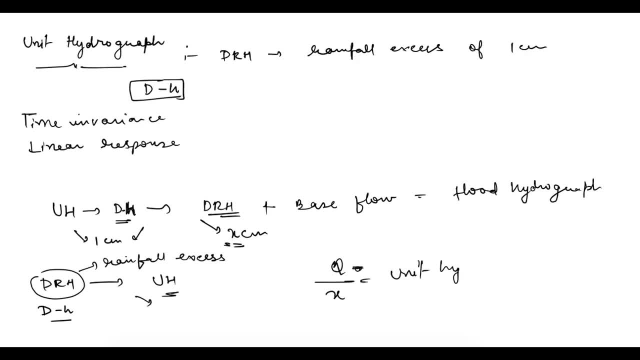 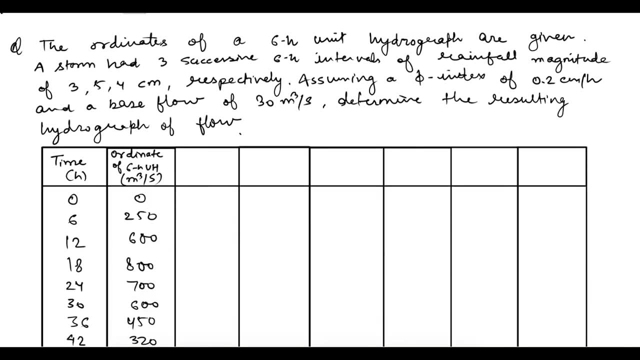 ordinates of unit hydrograph. So this we will understand better if we solve questions. So let's move on to questions directly. So it says the ordinates of a 6 hour unit hydrograph are given. The storm had three successive 6 hour intervals of rainfall magnitude of 3,, 5 and 4. 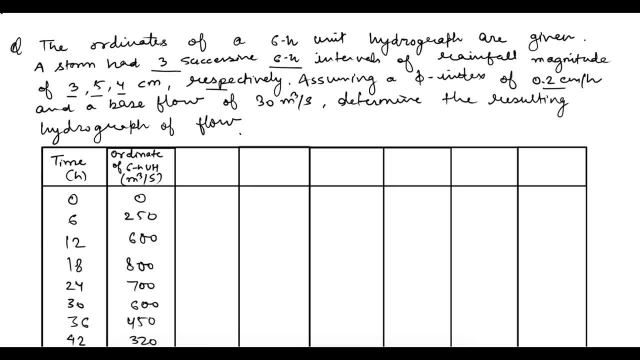 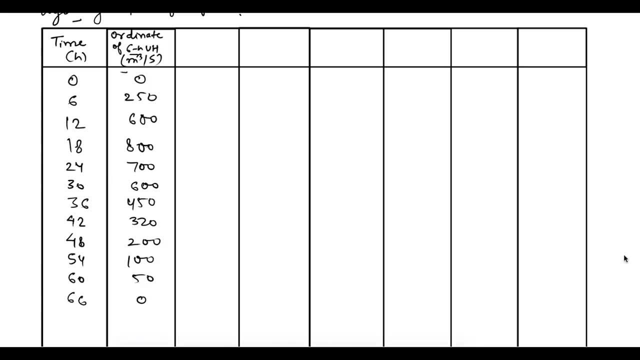 centimeters respectively, Assuming a phi index of 0.2 centimeters per hour and a base flow of 30 meter cube per second, determine the resulting hydrograph of flow. So here we have been given this time versus ordinates of a 6 hour unit hydrograph. So this is given to us. So in general, 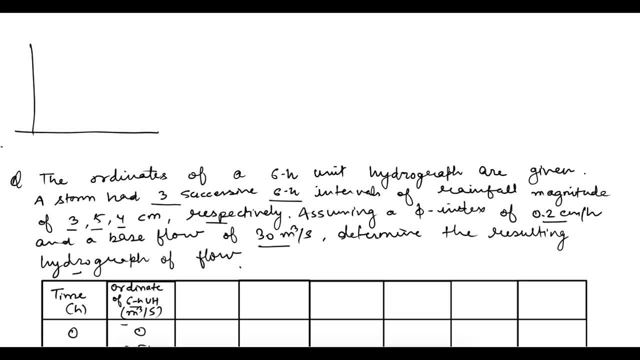 what we are doing here. let's say: this is your unit hydrograph ordinates And we have been given this rainfall. So rainfall data is given that three successive 6 hour intervals rainfall have happened. So that is from 0 to 6 hour. 0 to 6 hour there was a rainfall of 3 centimeter and from 6 hour to 12 hour there. 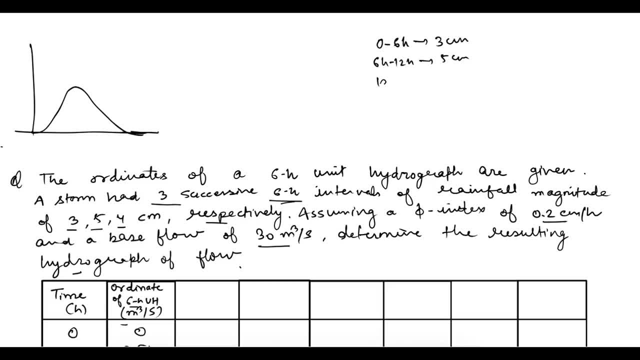 was a rainfall of 5 centimeter and from 12 to 18 hour there was a rainfall of 4 centimeters. So like this it is given Now this is the total rainfall. out of this total rainfall Some losses would be there. So for that losses, for those losses, phi index is given, that is 0.2 centimeters per hour. 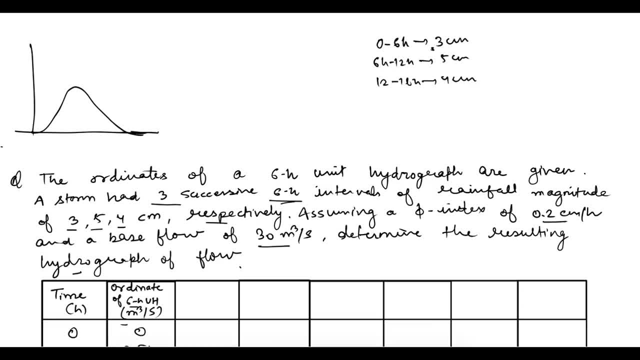 And what is the duration? Duration is 6 hours. So the loss, total loss, would be 0.2 into 6, that is, 1.2 centimeter. Here also 0.2 into 6 and here also 0.2 into 6.. We are taking the losses in all three of. 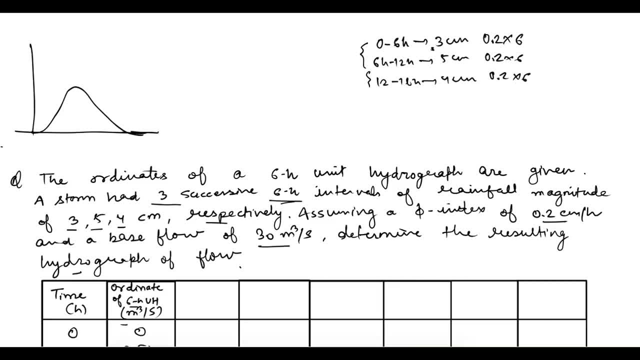 the rainfalls, because we are assuming These three to be separate. They are not related to each other, even when they are happening in the same catchment. We are assuming that these are not related to each other because we made this assumptions of assumption of time, invariance. So because of that, losses are happening in all these. 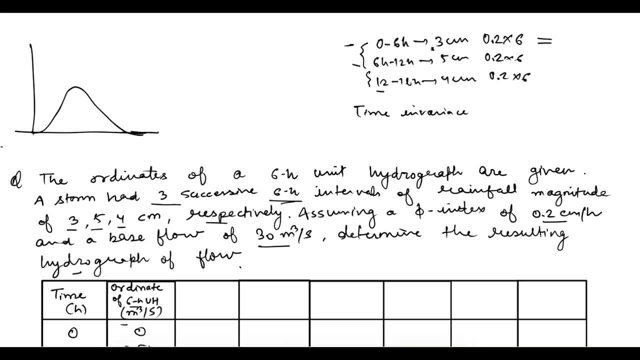 three rainfalls, Rainfall intervals I mean. So the rainfall axis here would be 3 minus 1.2, that is 1.8 centimeter, and similarly 5 minus 1.2.. 3.8 centimeter and 4 minus 1.2, that is 2.8 centimeters. Now we have to obtain first the DRH and we have the DRH. 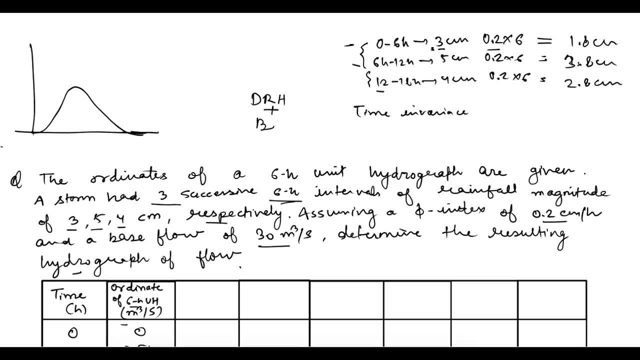 First, when we obtain the DRH, we will add the base flow to obtain our hydrograph. So, first of all, how to obtain this DRH? So for that, this is the data for 1 centimeter rainfall axis. So if, Let's say, if there is only 1.8 centimeter rainfall, So how will we do that? We will simply multiply these. 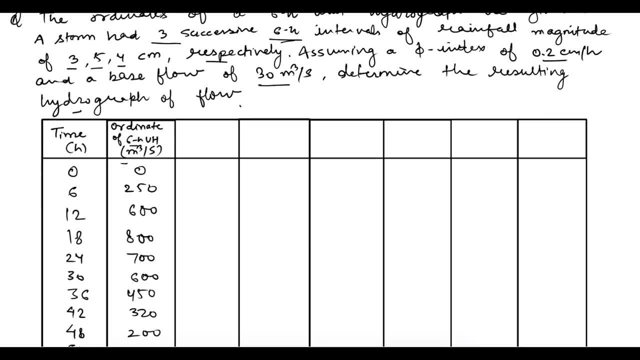 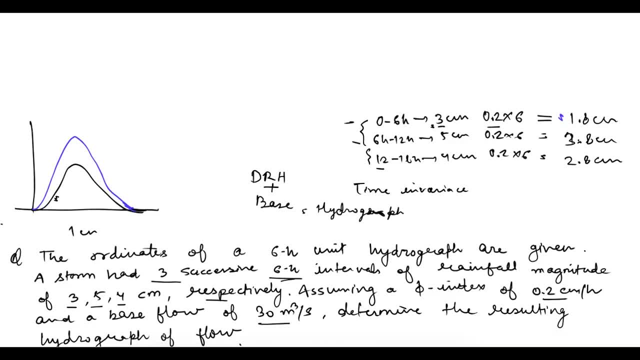 ordinates. So this discharge ordinates will multiply by 1.8. that will give us the DRH of 1.8 centimeter rainfall axis, Something like this. But here what is happening? after this 6 hours, next rainfall is starting from 6 hours to 12 hours. That is giving a rainfall axis of 3.8 centimeter. So let's say, if this is 0.. 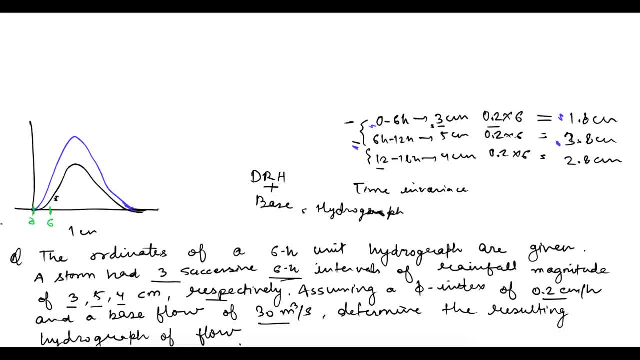 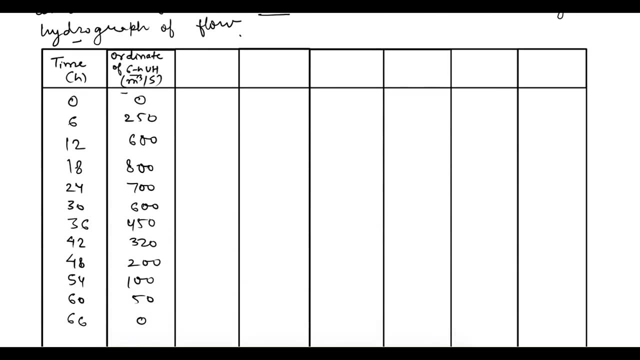 Then, from 6 hours, there is another rainfall which is giving a rainfall axis of 3.8 centimeters. So we will start the next series of unit hydrograph ordinates. So these ordinates, What we know for unit hydrograph, We will start from six hours. and so there we'll, and we multiplied with 3.8.. 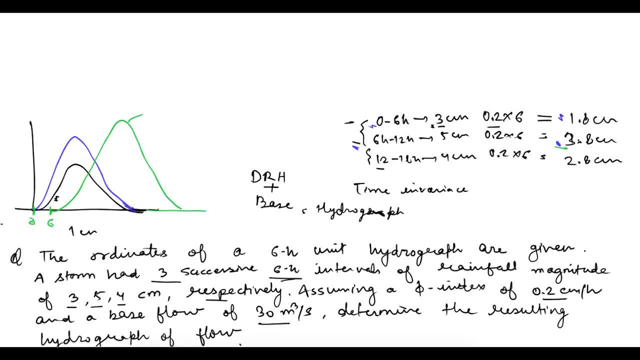 So that will give us a DRH Which, which will happen Due to 3.8.. Centimeters of rainfall axis, This is for 1.8.. Similarly, next one will start from 12 hours after this 3.8 is over. So here it will start from 12 hours. So that is again, we will multiply the unit. 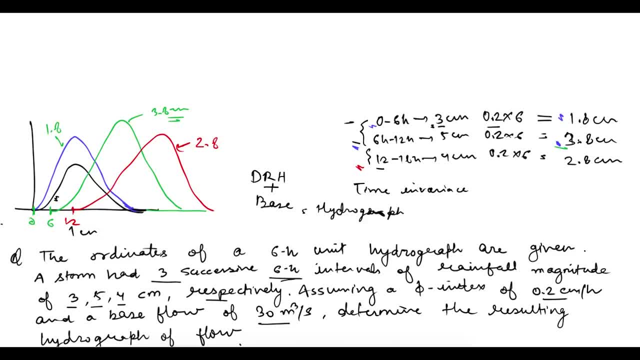 hydrograph ordinate by 2.8, by lagging it by 12 hours. So that way we will obtain the separate three. Then for the final one, for the cumulative effect of all these three, we will do the addition of all these three, I mean the ordinates of all these three, So like this we will get the actual. 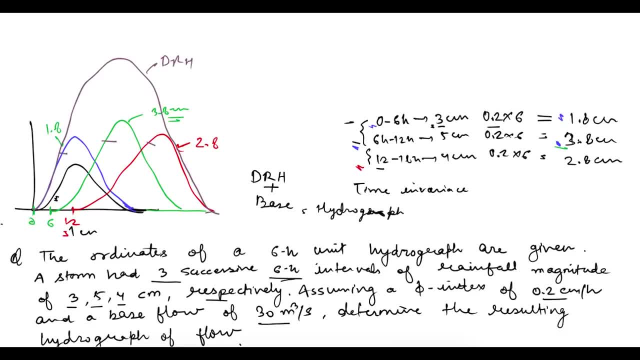 direct runoff hydrograph for this complete overall flow, that is, 2.8 plus 3.8 plus 1.8 centimeter, And in this we will add the base flow to obtain our hydrograph. So this is what we are going to. 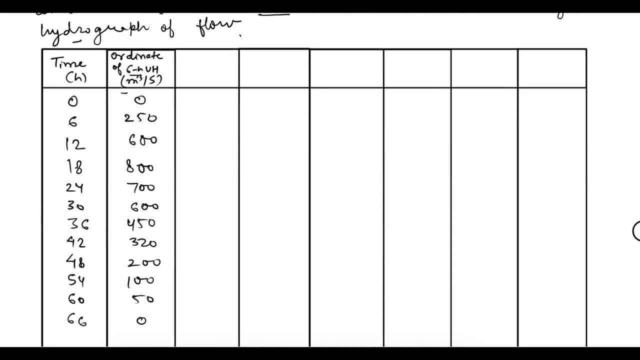 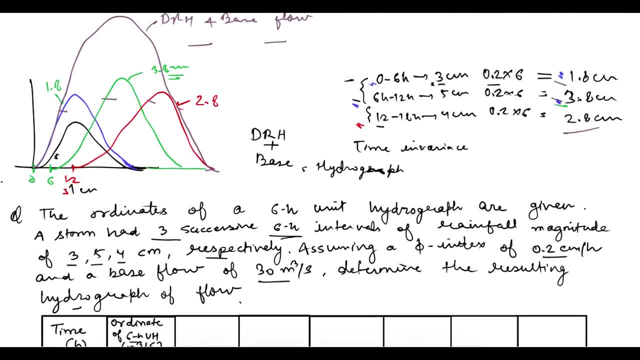 do here. So I have just explained. now we can simply do so here. ordinates are: given rainfall axis, we have calculated 1.8.. 1.8 cm, 3.8 cm and 2.8 cm. So the first step is to multiply this unit hydrograph ordinates. 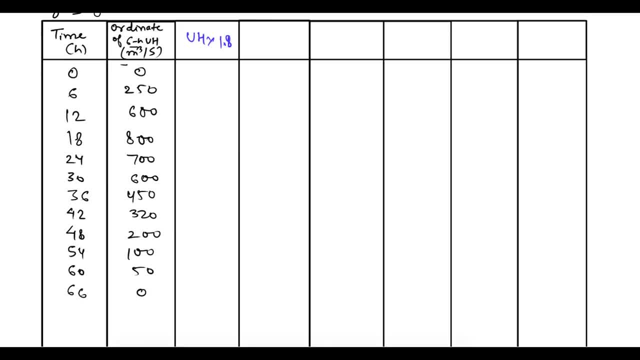 by 1.8 cm, because the first rainfall is of 1.8 cm rainfall axis. So the ordinates with come out as we do this, multiplicating 0,, 450,1080, and this is 1.40.1260,10802.. This 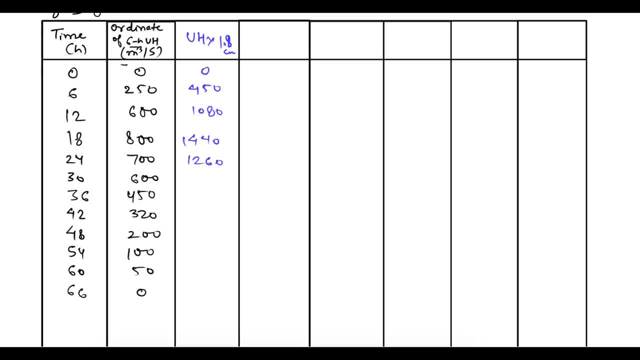 is this all going to come out as Altinnita divider into 0.. And finally, we will import some各位, reopen the symbol And then for the grid, if it looks gone, Kinder, eight, zero, eight, one zero, and then five, seven, six, three, six, zero, one, eight, zero. this is 90 and again. 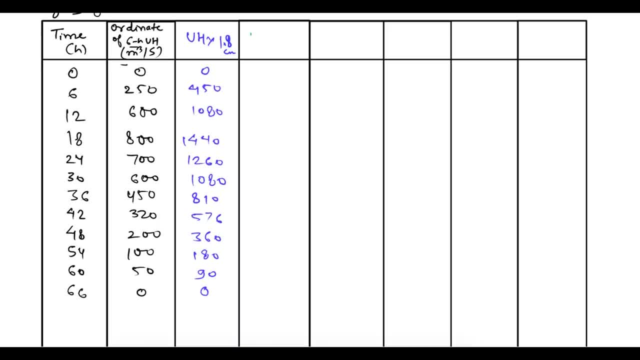 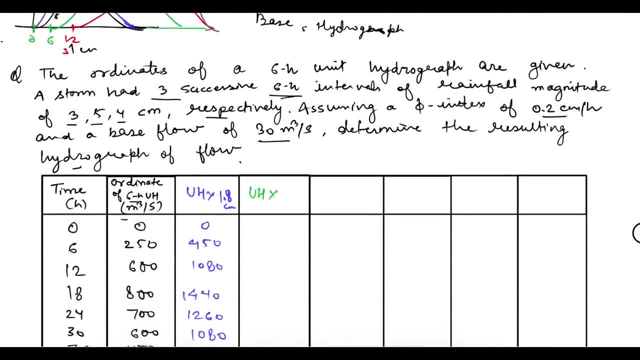 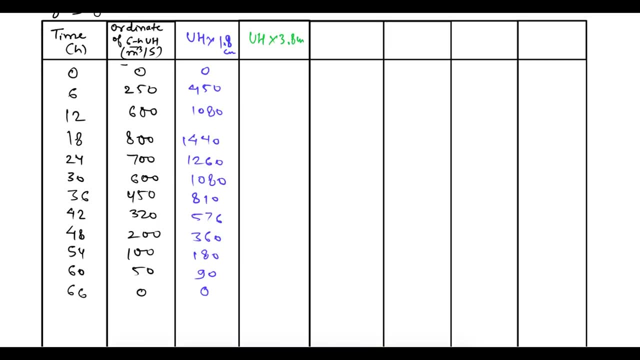 zero. this is the first. now the second rainfall in this unit hydrograph ordinate will be multiplied by how much. the second rainfall is of 3.8 centimeter rainfall axis. so this unit hydrograph ordinate is multiplied by 3.8 centimeter. but it will start from six hours, so we will start from. 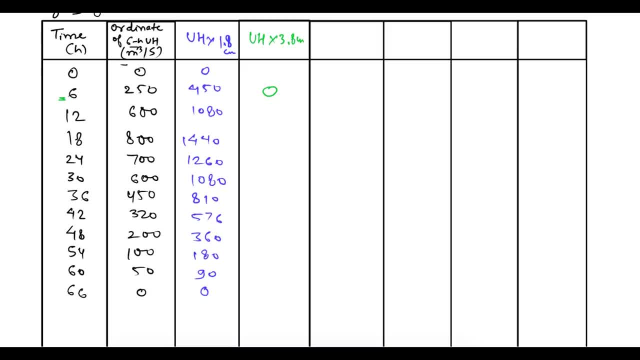 six hours, so it is at six hours it is zero. and then this 250 is multiplied by 3.8, and that will give 950, and 600 multiplied by 3.8 will give 2280, then 800 multiplied by 3.8 will give 3040, and 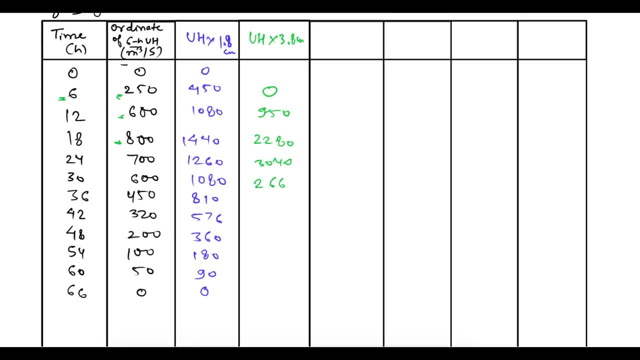 we can calculate for other. so next is two six, six zero, then we have two, two eight zero and one seven, one zero. one, two, one, six, seven, six zero, then three eight zero, one nine zero and the next is zero. so here the duration is exceeding, so here this is next, that is, for it is coming up to 72 hours. 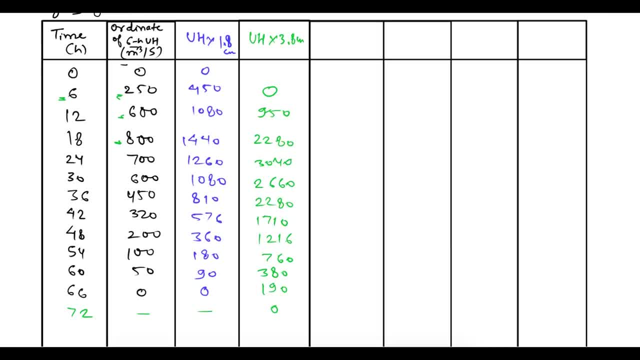 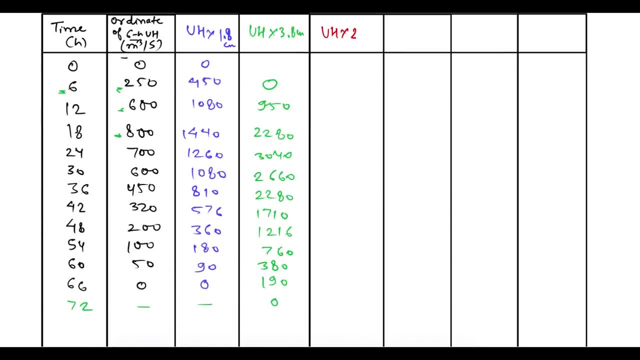 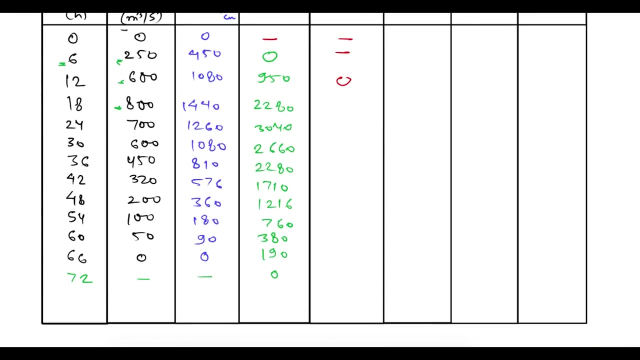 so that is the next one. now the third one, that is, unit hydrograph ordinate multiplied by how much. it was 2.8 centimeter. so this last rainfall will start at 12 hours. so here it will be zero. here it is nothing. similarly, here for first two, nothing is there. so it is starting at 12 hour. so 2.8 multiplied by 250. so 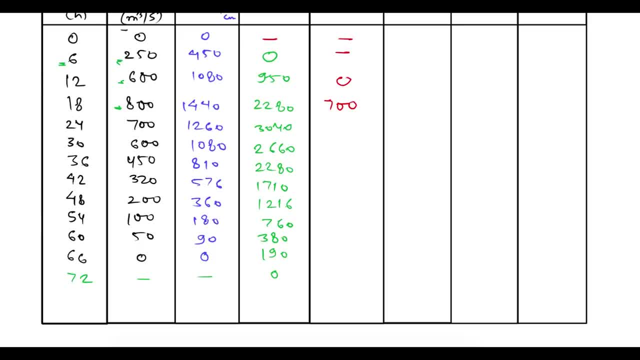 that is 700, and then 600 multiplied by 2.8, so that is one, six, eight zero. and similarly we can do for others: two, two, four zero, then one, nine, six zero. one, six, eight zero. one, two, six zero, eight, nine, six, then five, six zero, then two, eight zero corresponding to this, and after that one, three, eight, two and six. 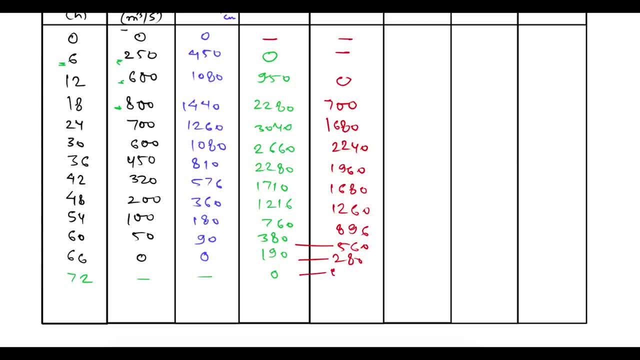 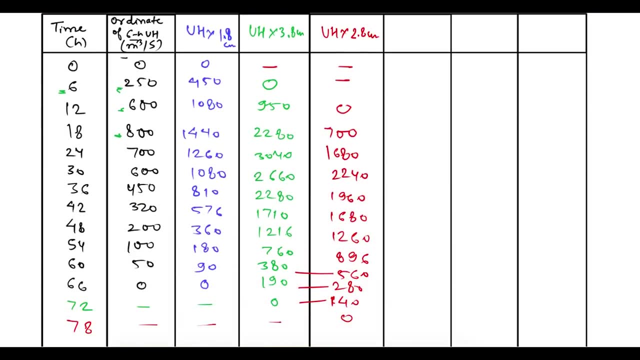 eight zero, And after that 1,, 4,, 0 and then 0. So here one more duration is coming, that is 78 hours. So all three have. we have done the summation. Now we can obtain the direct runoff hydrograph- direct runoff hydrograph, which will be the summation of these three. 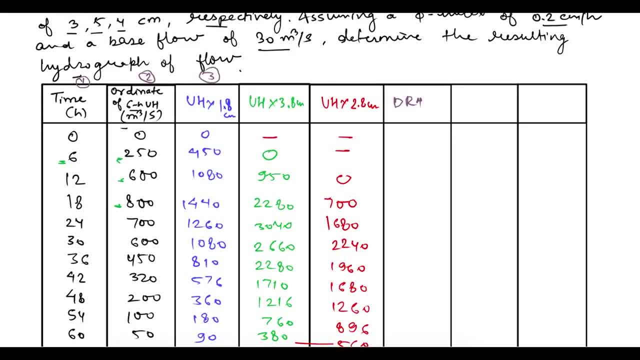 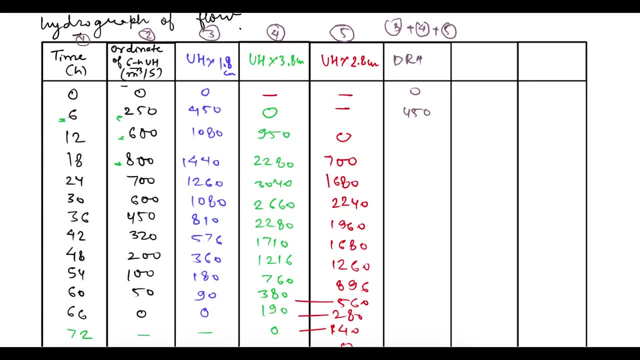 So if it is 1, 2, 3,, 4 and 5.. So this is a summation of 3 plus 4 plus 5.. So that is here. it is 0, then 450.. Then this is 1, 0, 8, 0 plus 950.. That is 2, 0, 3, 0.. And then similarly you can do for rest, That is 4, 4, 2, 0. 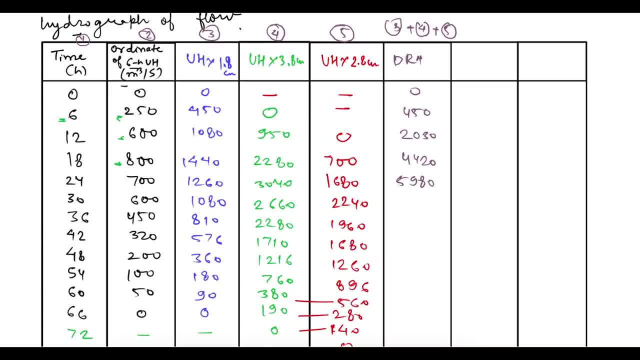 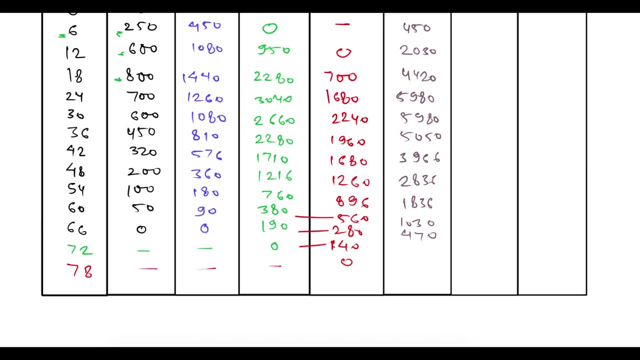 Then there is 5,, 9,, 8, 0.. Then next is also 5, 9,, 8, 0.. And then 5, 0, 5, 0,, 3, 9,, 6,, 6,, 2,, 8,, 3, 6,, 1,, 8,, 3,, 6.. And after that 1, 0, 3, 0,, 4,, 7, 0.. Last one is 140.. And then it is 0. 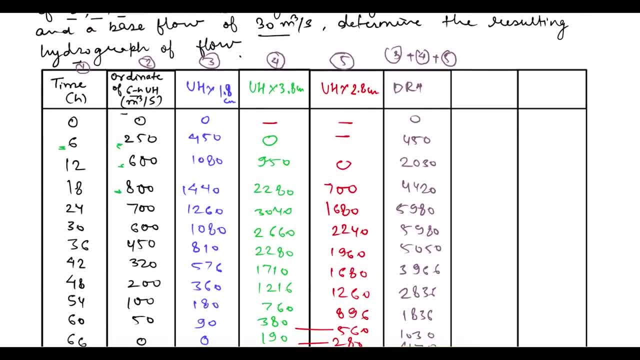 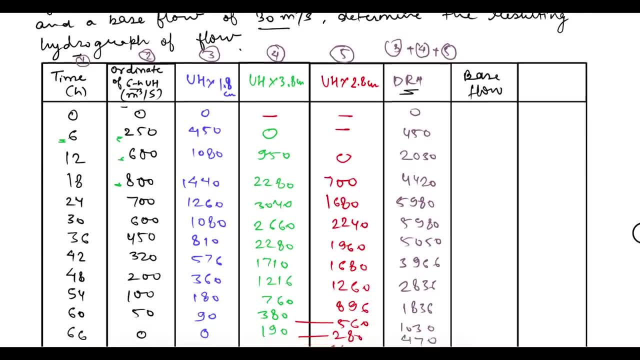 And then we have base flow. base flow is given in question these. this one is the ordinate for direct runoff hydrograph. now we have to, if you have to obtain the hydrograph, so for that we'll have to add the base flow also. so that is 30 is given for all. 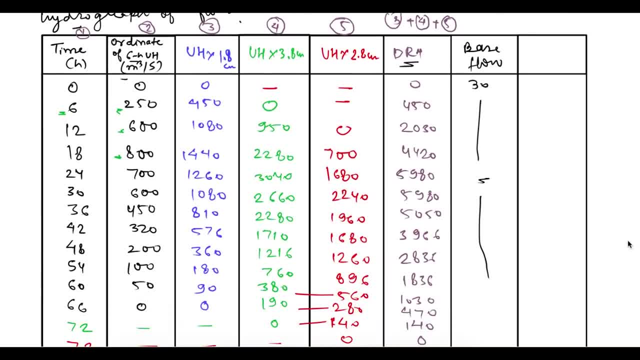 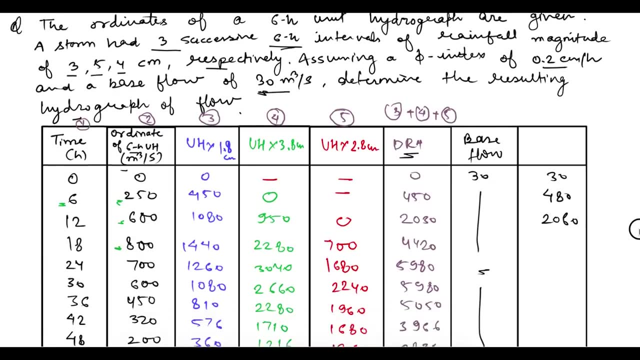 these same value. so just add the 30 here, so it is 30, then it is 480 and 2060. similarly you could do for the rest. so this is this is a standard theoretical question. I just wanted to show the steps. later we solve the gate questions that. 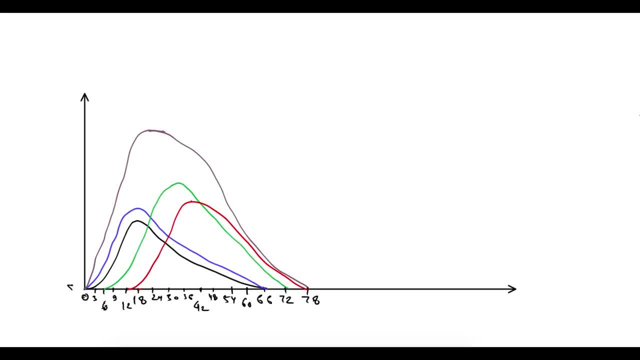 will be. I mean, that will be of shorter duration. so this is what I, what I had shown earlier. this is for unit hydrograph, then this one is for. this one is for 1.8 axis, this one is for 3.8 centimeter axis and this one is for 2.8. 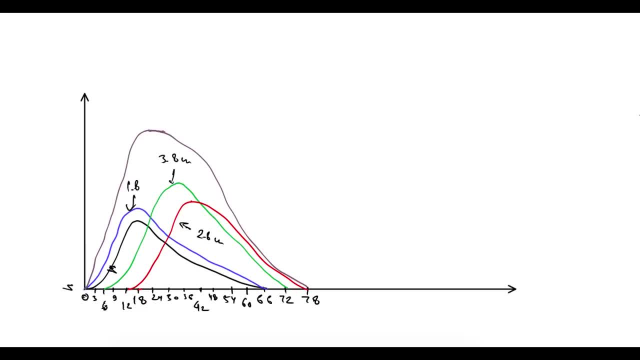 axis, and this one is for 3.8 centimeter axis and this one is for 2.8 centimeter rainfall axis, and then we do the summation to obtain the direct runoff hydrograph and after that we have done the summation of the base flow to: 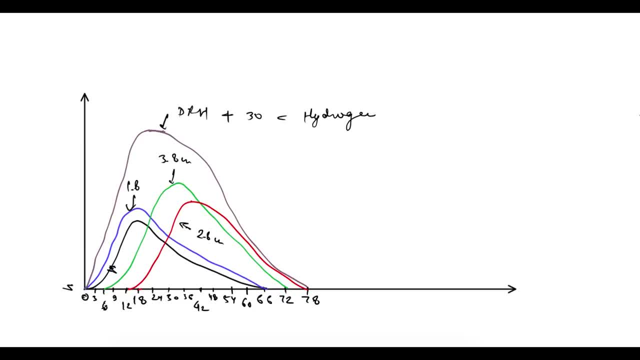 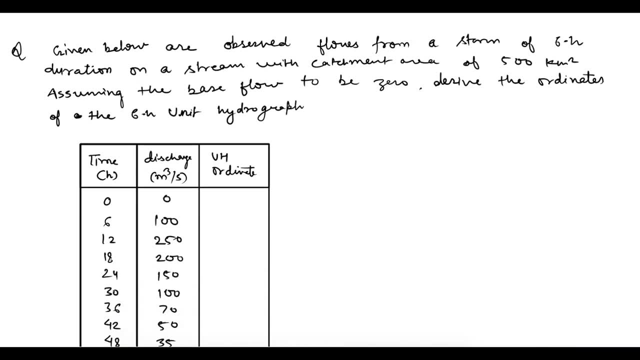 obtain the hydrograph. these are the steps we have followed here. so now let let's see the diff. I mean opposite kind of question where we have to obtain the unit hydrograph from direct runoff hydrograph. so it says: given below are observed flows from a storm of six hours. 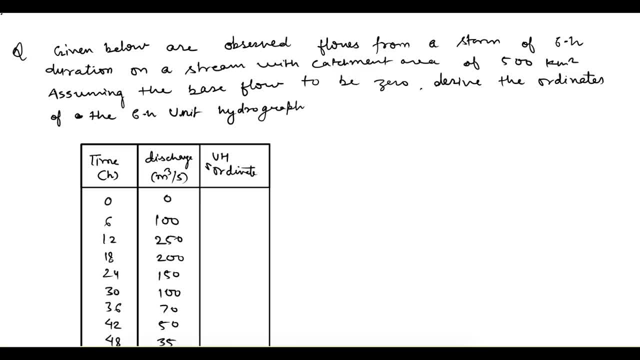 duration on a stream with catchment area of 500 kilometer square, assuming the base flow to be zero, derive the ordinate software of the six hour unit hydrograph. so area of the catchment is given, that is, 500 kilometer square, duration is given as six hours and we have been given this time versus discharge data. so 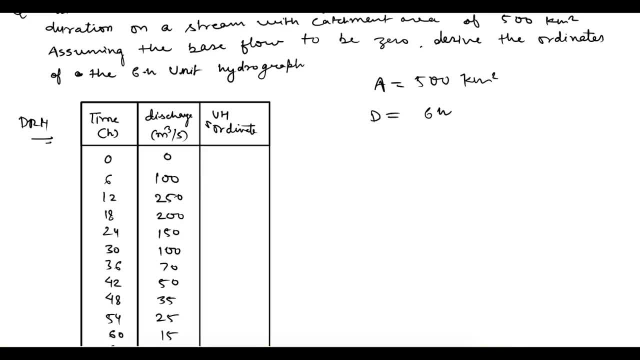 this is nothing but your direct runoff hydrograph data. now we have to obtain the unit hydrograph from that. so if you have a unit hydrograph and you have to obtain, or you might have to get, at least some additional amount of link to call that редact time, so say, let's say so here. So, as you can see, this is a 300 meter. 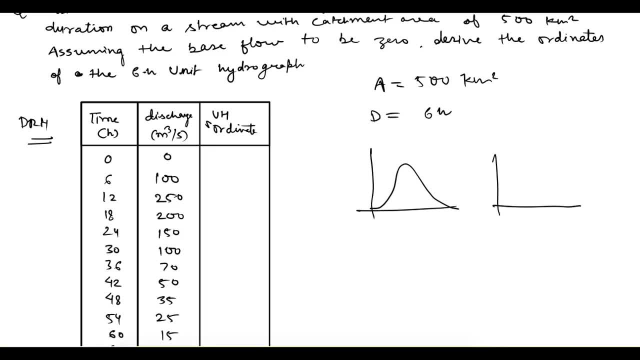 time for a hydrograph. and if you remember that, we saw that if this is your direct runoff hydrograph and corresponding to that, we can plot a plot, an effective rainfall hydrograph. it is Er H, this is Dr H, so we saw that this is Q versus time. so the area of this hydrograph, area of this hydrograph tips, 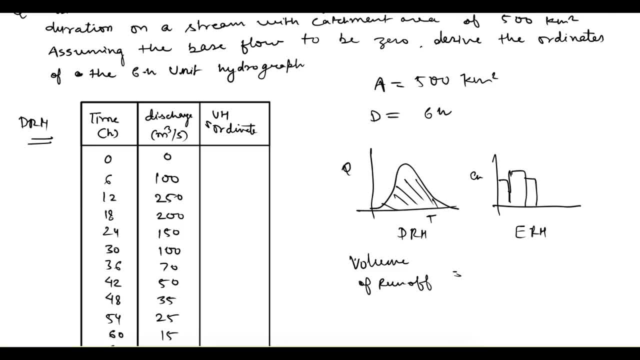 and the- I mean this is the units here- are centimeter per hour and here this is again the time unit. let's say this is also in hours. so here we will get the rainfall in centimeter, and if we multiply it by the area of catchment, so 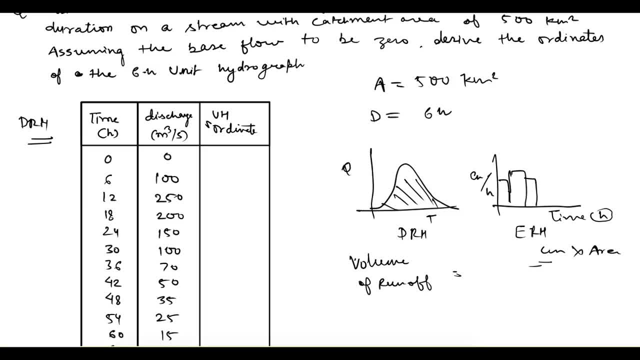 that also gives what volume of runoff. so that is rainfall axis, rainfall axis into area of catchment. that means here what all we know, we know the- I mean this data time versus discharge. so similarly we can plot such Hydrographs and we know the area of catchment. so if we can find out the area of this hydrograph and will 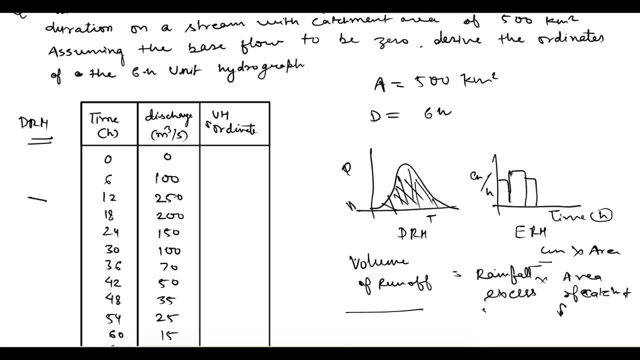 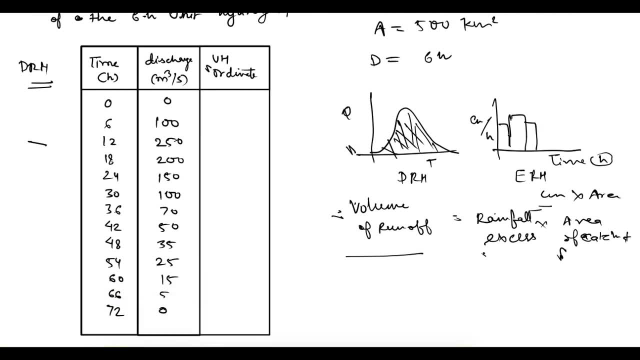 divide it by the area of catchment, so that will give us the rainfall axis, because Ayuri of hydrograph is gives what volume of runoff. volume of runoff by volume of catchment, because of which Seward is not exactly able to of divided by rain area of catchment, will give us rainfall axis. that is, volume divided by area. 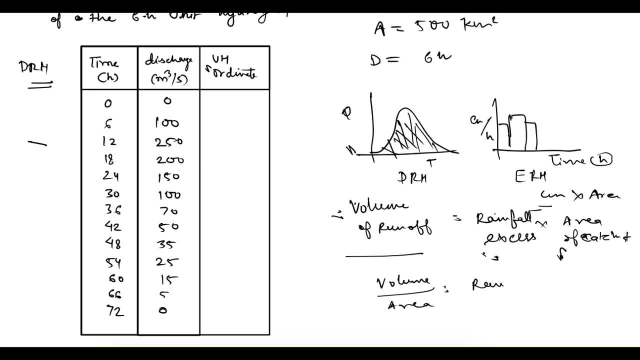 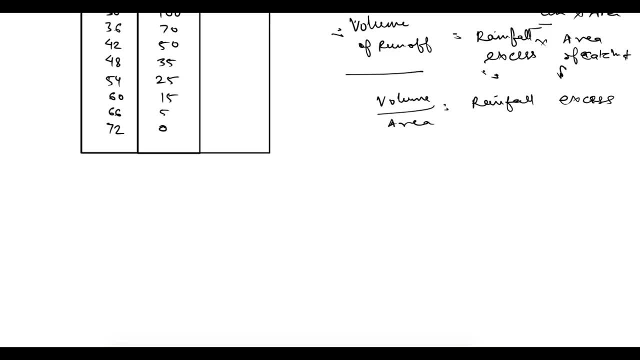 will give us the depth of rainfall, and that is nothing but your rainfall axis. so just that: we have to find out this area of hydrographs here. that is the important step. so for that, if nothing is given in the question, then you are going to follow the trapezoidal rule. so here, data is given. 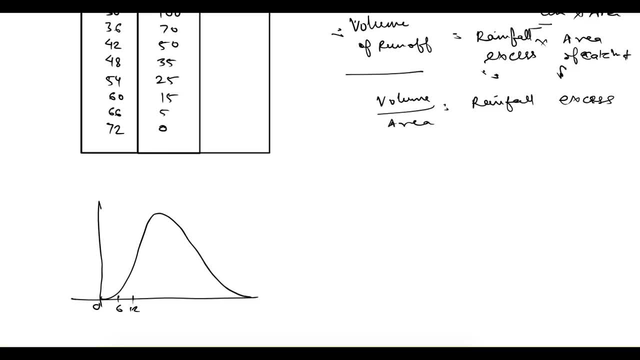 that is 0, 6, 12, 18, 24, 30, 36, so on. so we can divide it into small strips and then we can apply this trapezoidal rule, or you can find out the area individually also, but that will take time. so 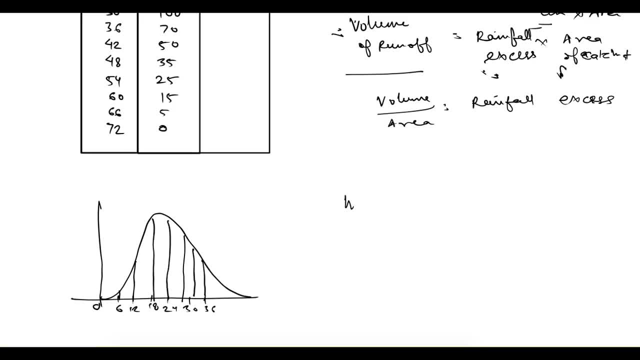 simply, you can apply the trapezoidal rule so that is delta h upon 2 x naught plus x n plus 2 into x 1 plus up to x n minus 1, so that we can apply to obtain the area under this hydrograph area of curve. we can say: so that is delta h here, the difference we are taking. 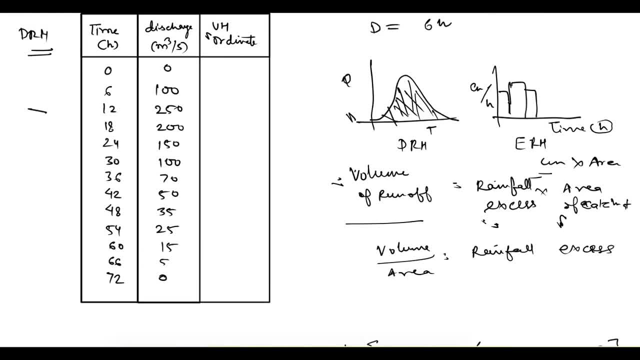 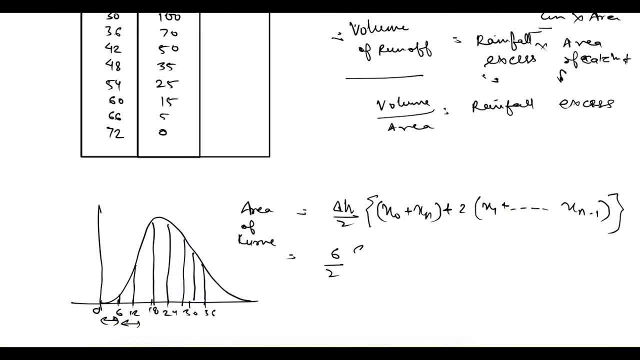 is 6 r, so that i mean we know because the value at every 6 r, so that's why we are taking so h. this delta h is 6 divided by 2 x naught plus x n, first and last value. both are 0. 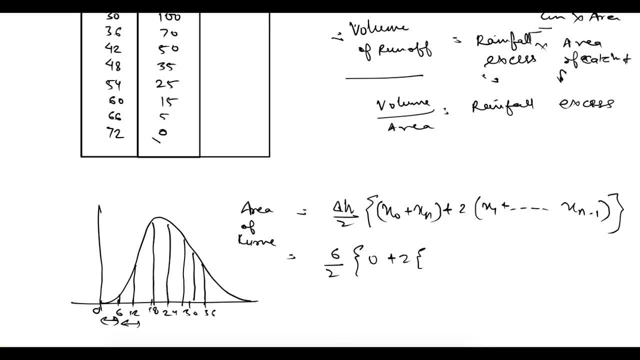 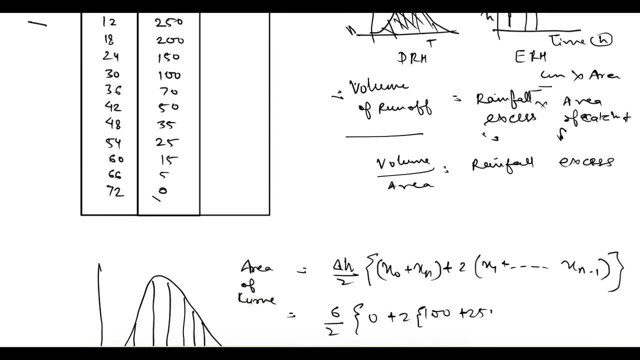 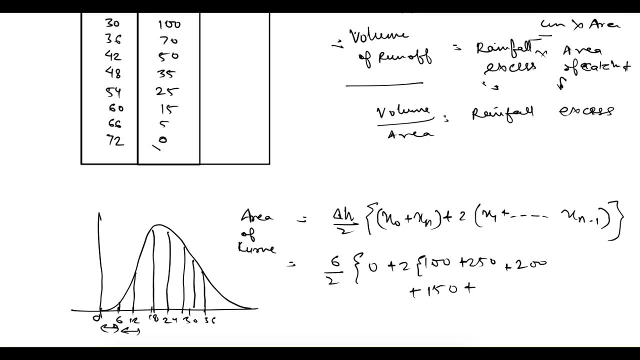 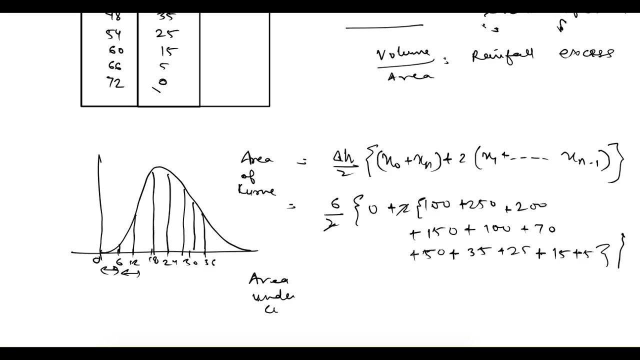 so that is simply 0 plus 2 into rest of the values. so let's write that that is 100 plus 250 plus 250 plus 200 plus 150 plus 170, 10 plus 350 plus 150 plus defence, 15 plus twenty-five plus fifteen plus five. so here these two will cancel out. so area of curve. 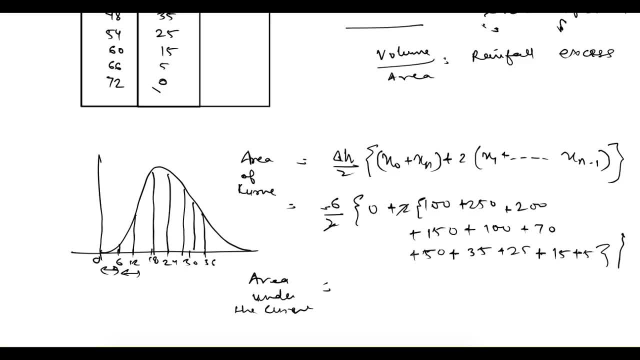 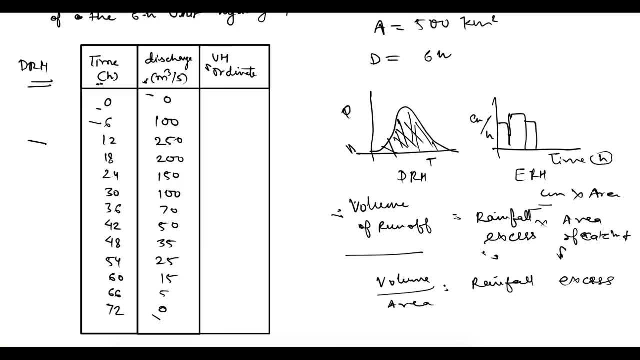 area under the curve. we can say area under the curve is equal to six. so here the unit of time is in hours and the unit of discharge is in meter cube per second. this is in meter cube per second. in meter cube per second this is in hours. so time also will convert in in second. so that is 6 into. 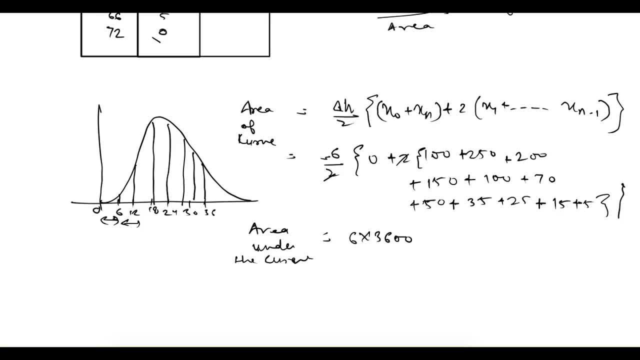 3600 because because it was in hours, so 3600. if you multiply it with so, if you solve this, if you multiply with this rest of the value, then total it comes out as 21600 meter cube. so that is what that is. what we have obtained is volume of runoff. area under the curve is equal to volume of runoff. 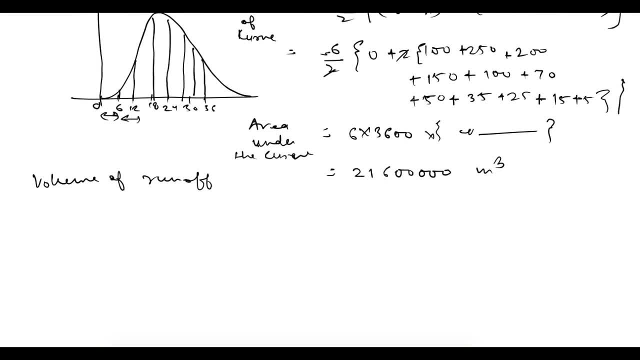 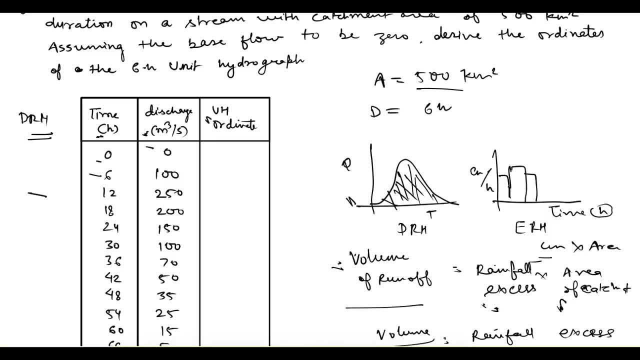 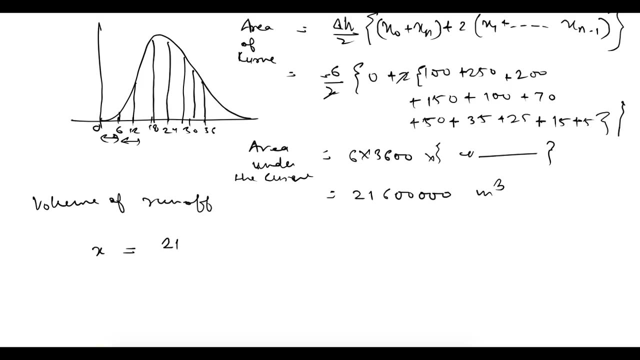 now we can simply obtain the rainfall axis by applying this formula: volume divided by area of catchment. so area of catchment is given to us that is 500 kilometer square. so that is rainfall axis. x is equal to volume 216, x is equal to volume 216.